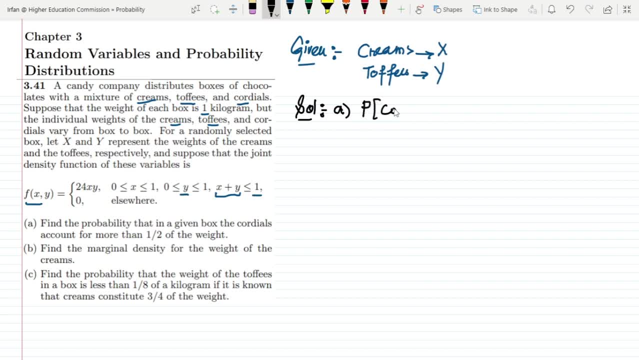 To find the probability that cordials are what Their weight is, more than 1 by 2 or half of the weight. So that is greater than 1 by 2.. But here we can very easily see that the joint distribution or joint density function doesn't encounter the cordials, It is only including the weights of 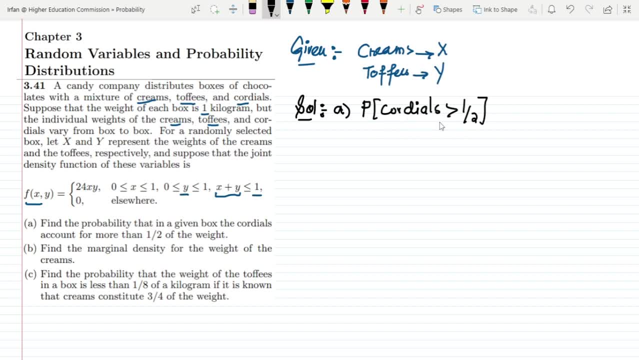 the creams and toffees. So therefore, if the weight of the cordials is greater than or equal to 1, then 1 by 2.. So it means the combined weight of x and y will be less than 1 by 2.. So what I can do, 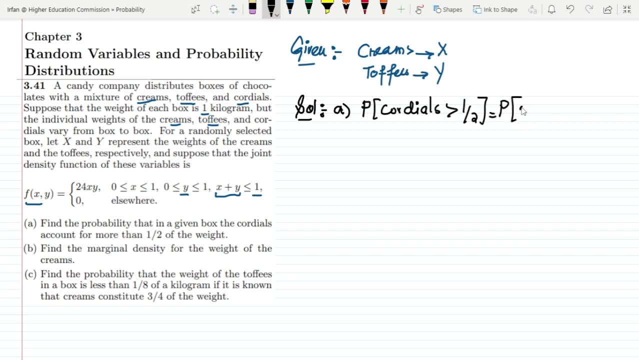 here is that. I can here very clearly see that it will be: x plus y will be less than or equal to 1 by 2.. So it must be understood in this way. So it will be like this one. So now, in order to find: 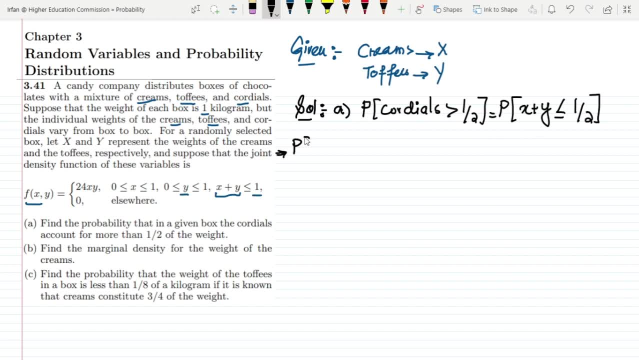 this probability. what do we have to do? We have to find the probability that x plus y is less than or equal to 1 by 2.. So we can use here for this addition, we can very clearly see that this is a continuous function, So for it we can use the integration. So for integrating it. 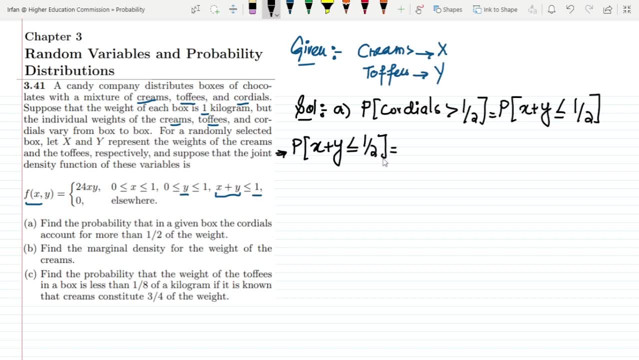 we have to use different ranges of x and y. So if the y range is from 0 to 1 by 2. So the range of x would be from 0 to 1 by 2.. So the range of x would be from 0 to 1 by 2.. So the range of x would be. 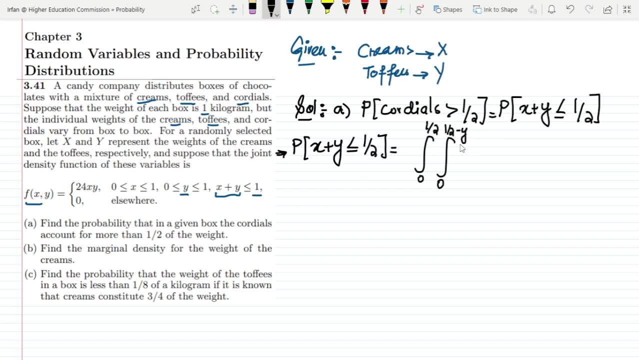 from 0 to 1 by 2 minus the weight of a y, So this will be subtracted from 1 by 2.. So now writing the function here, and that is 24 x- y, and also integrating it with respect to x, and integrating 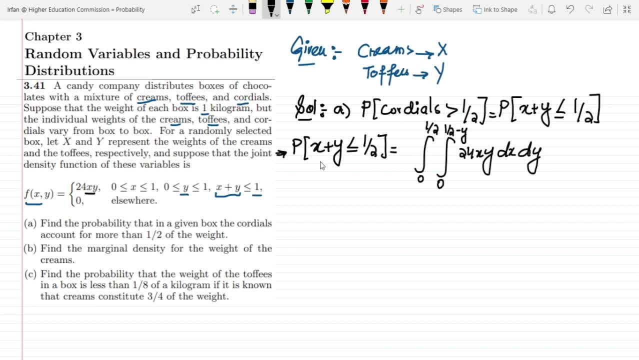 it with respect to y as well, Because now we have been adding the two functions, So therefore I have to add them together by using the integration which is for the continuous functions, Now here, 0 to 1 by 2, and integrating it first with respect to x. Okay, this part. So what will we get? 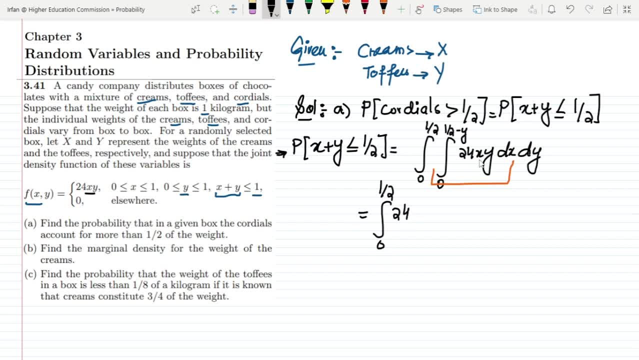 Here we will get 24, and here this is with respect to x, So x square divided by 2, and here we will have y. Okay, and also it will be from 0 to 1 by 2 minus y, and integrating with y is left, So now it will be 12.. Okay, and also, putting these values, what I will get Here, I will: 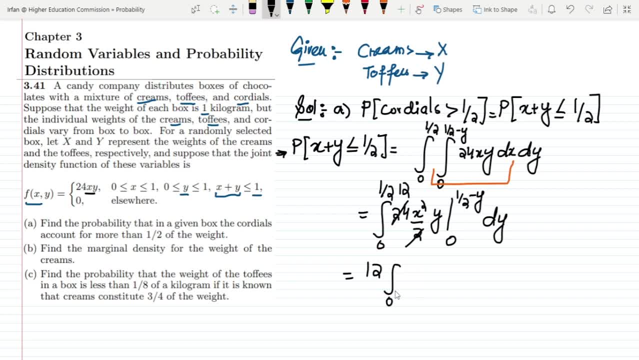 get 12 will be outside, and here it will be 0, 1 by 2, and putting these ranges here, I will get 1 by 2 minus y whole square, Okay, and also this y here and then dy, Okay. so this is for. 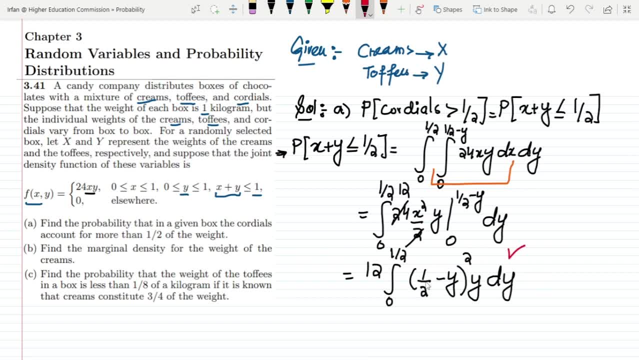 this one. Okay, this is the function we have got Now, after it, using the integration by parts. Okay, so, integration by parts for this one, for dy, at the end, putting all the limits and all the values, what I will get at the end? the answer of it will be 1 over 16.. You can use here integration by parts. 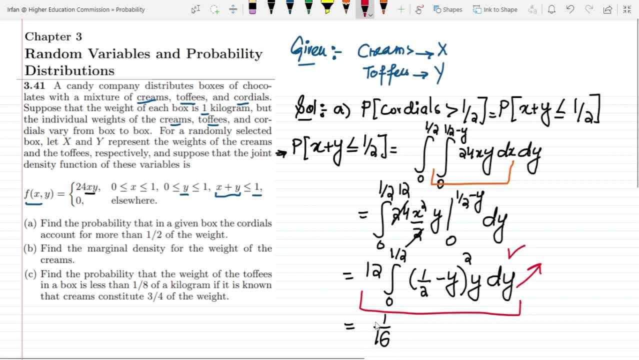 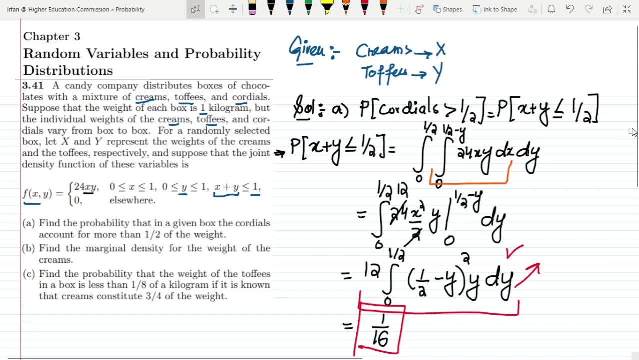 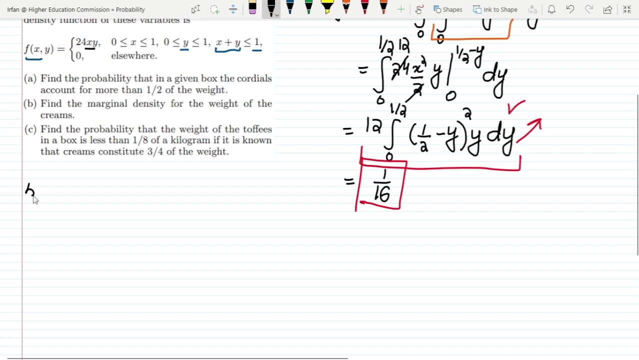 by yourself and see that the answer of it will be 1 by 16. and that is what. that is the solution of partition. Okay, so I hope you have understood it Now moving somehow downwards, Okay, and now seeing part b of my question, Okay, so what is part b? Find the marginal density for the weight of the creams. 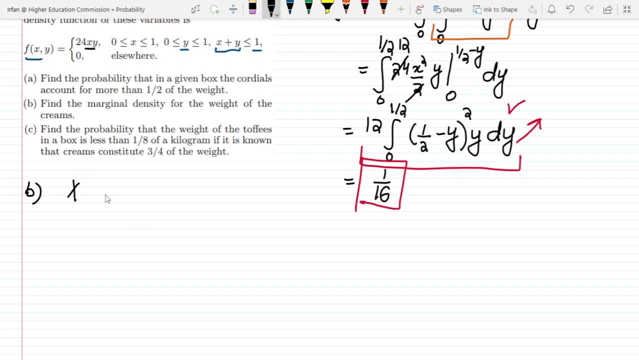 Okay, so weight of the creams are represented with x. Okay, we have seen that, and for it, let me find the marginal density for it, and let me represent it with g of x. Okay, so let me find it out. and finding it out, I have to define the limits for the function which is here, So it will be from 0 to word for any value. 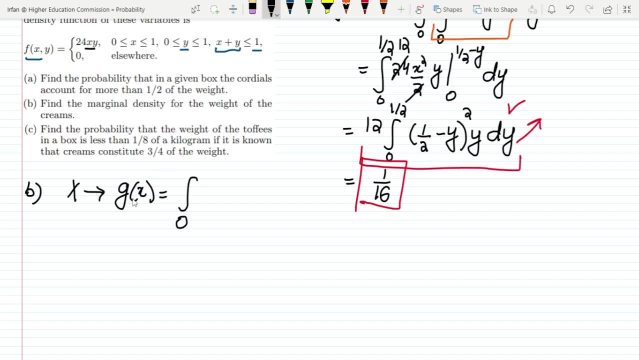 which will be less than 1 kg, because if it will be composed of the cream, the other items will also be included. So those would be: weight of the cream will be subtracted from 1, which is the 1 kg. So therefore it will be from 0 to 1 minus x the quantity of the creams subtracted from the 1 kg. 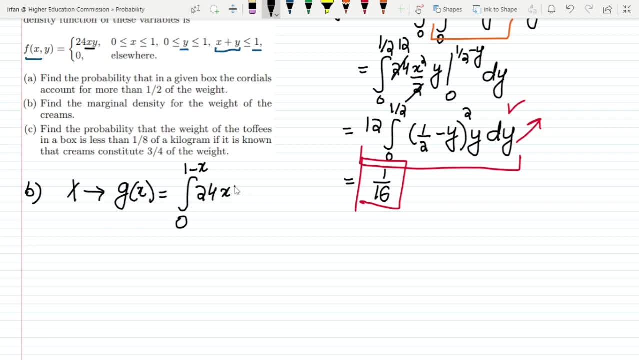 Okay, so now writing here, the value is 20.. So now we are going to get 24 x y, and now again integrating it with respect to dy. Okay, so now using it and what I will get? here I will get 24 x, and here this will become what y square divided by 2, and here 0, 1 minus x. 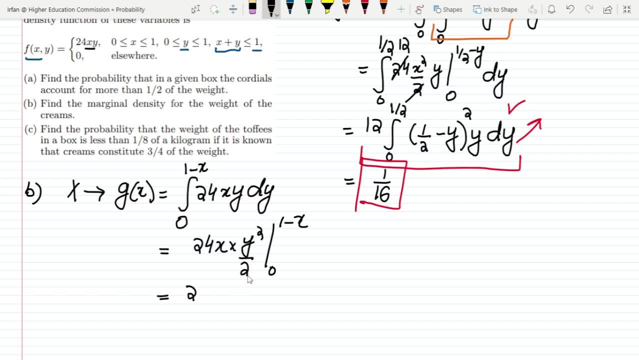 Okay, so now it will become 24 and this, this will become 12 here. So I will get here 12. And here 12x, and putting 1 minus x and 0 here, so ultimately I will get 1 minus x square, and that is. 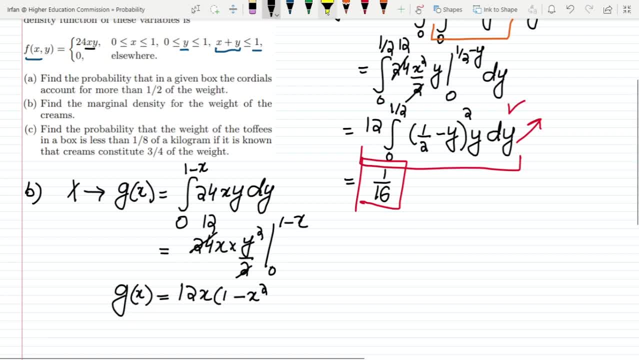 for the marginal density for x or weight of the reel. So that is what we have found out. This is the answer of part b of my question. So also the range of x will be here what we have to define, the range of x as well. So the range of x will be greater or equal to 0 and it will be restricted. 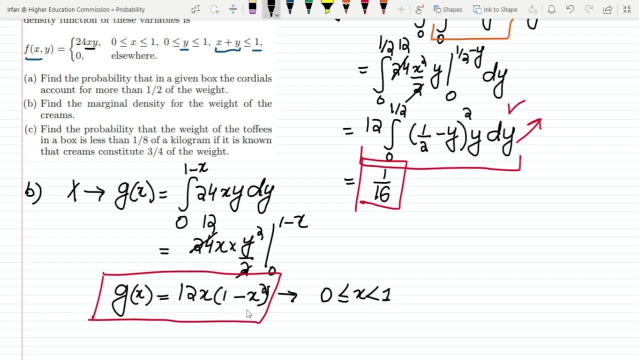 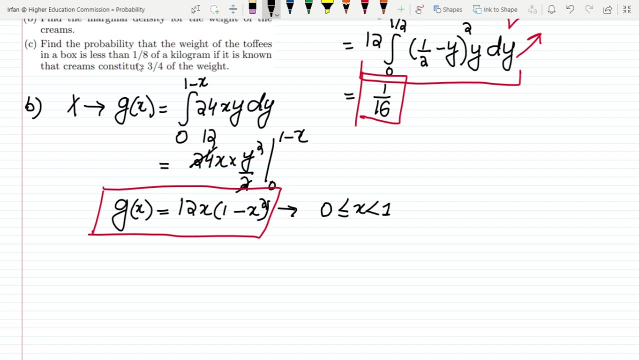 less than 1, because all other items will also be included, So I am not making it equal to 1.. So that is the solution of part b. Now, moving to the part c of my question, Find the probability that the weight of the toffees in a box is less than 1 by 8 kg. So let me first write the given. 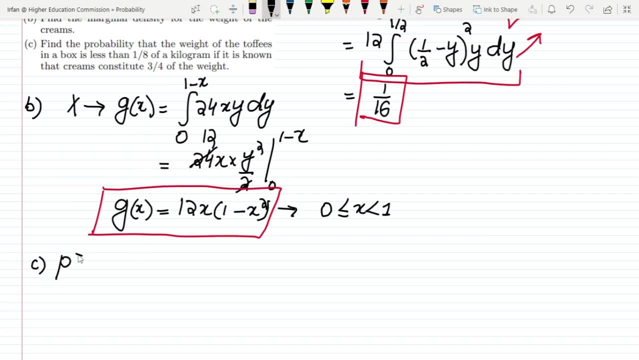 data. here We have to find the probability that the weight of the toffees in a box is less than 1 by 8, and we have seen that the weight of the toffees were represented with what, That those were represented with y and. 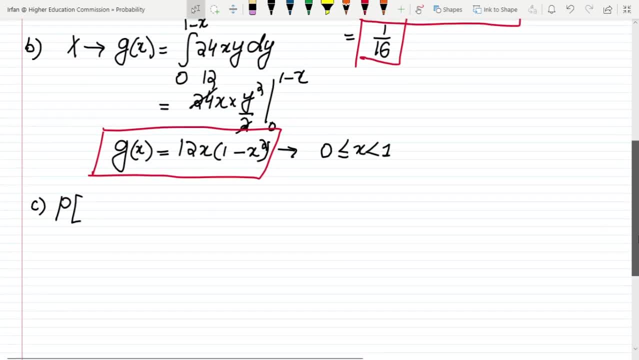 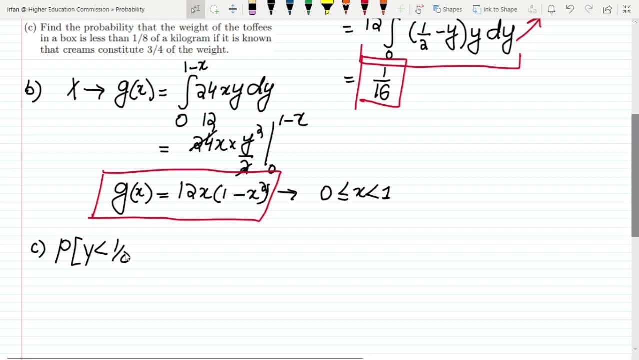 creams were with x. So therefore the weight of y is less than 1 by 8 kg. If it is known that creams consume 3 by 4 of the weights, and given here is that creams which are x, these are of 3 by 4, we have to find it. 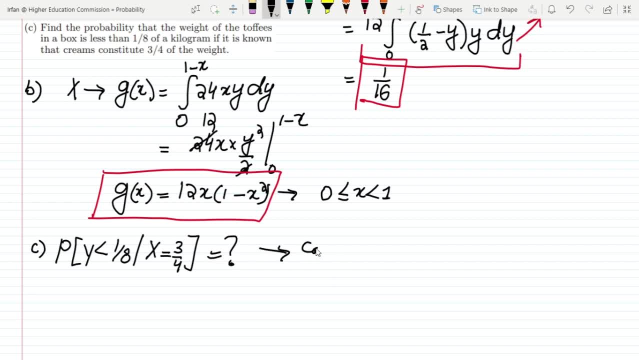 out, And we can very clearly see that this is the case of a conditional probability, Because one probability has been given and on the basis of it, we have to find the probability of another item, which is the case of the conditional probability. Now, using it and 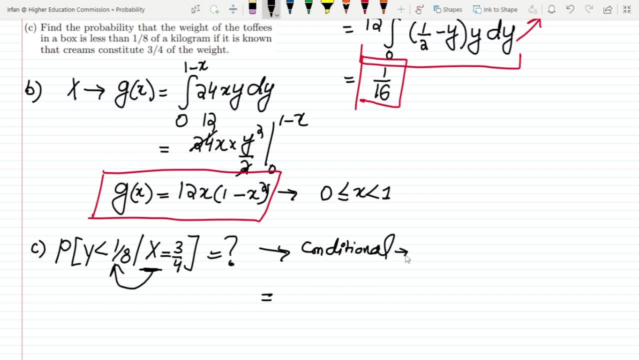 finding it out. the formula we have already known for the conditional probability is the p, x and y divided by the probability of x. Okay, y, x, because here you can see that this probability is given. So this will be written here and those two items has been included here as well. Okay, so we can see. 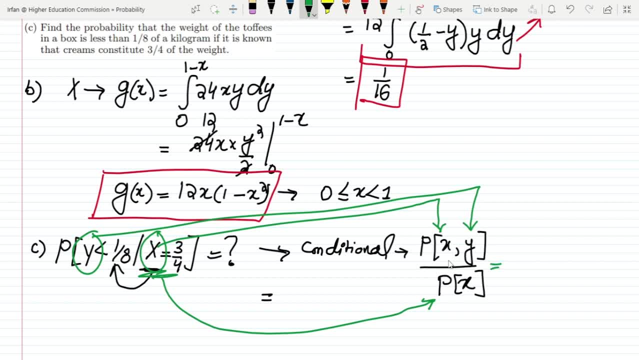 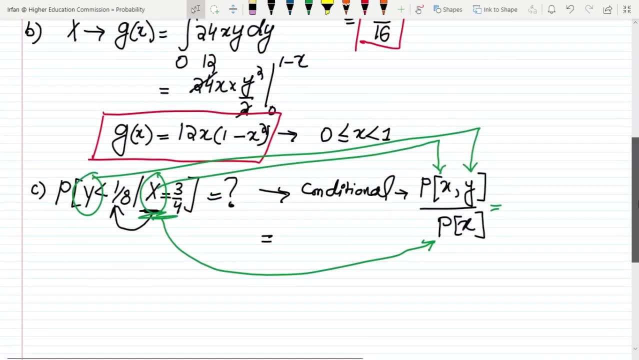 it here as well, Now writing their values. do we know the probability of the toffees in a box? Yes, This is the same thing which is already given in the question. We can see that this is word. This is already given here. This is 24 x- y. Okay, give it to me, Let me write it here, which is 24 xy. 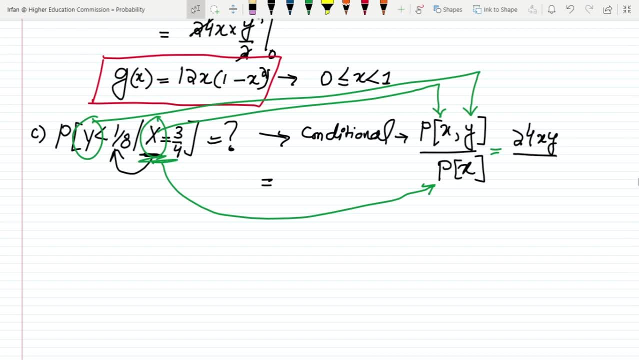 Okay, and the probability of X, Do we know it? Yes, that is also the marginal density which we have here, and that is AB is 12 x1 minus X하고. we know x, y as the original dread, x as Professor Richter's query. So as and we need to use f combination. there is agged each part of f and each part of y. also оч y unique vector in the question which Call is F which is equal to y, or only which x, or log by x el? you know that in which photo? 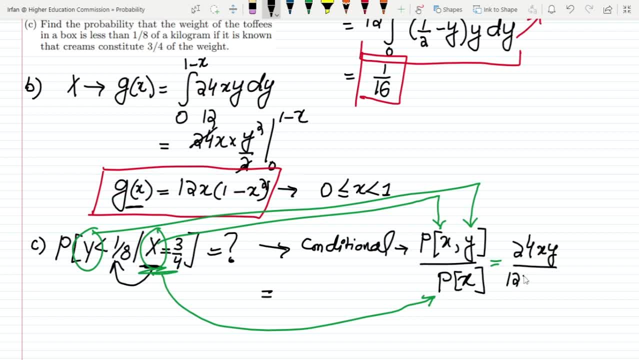 Here and that you can see. if you want to say that a equals natural cost is equal to or equal to F, confused with anything which becomes x minus x is and a quasi x. so 12 x 1 minus x square. okay, so these two will cancel out, this will be 2 and ultimately, 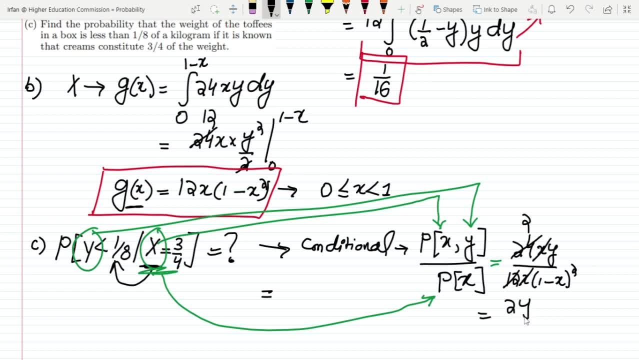 I will get what I will get: 2 y divided by 1 minus x, whole square. okay, so that is what. that is the formula for the conditional probability which is given here, and here we have to consider the ranges of x and y as well. so putting those values here, 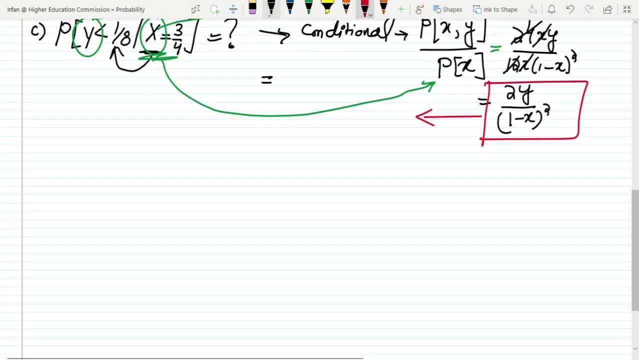 okay, so putting the values of x and y here, because the value of x is already given. so putting this 3 by 4 here, what I will get here? the probability that y is less than 1 by 8, such that x is equal to 3 by 4. okay, so here now putting the value of. 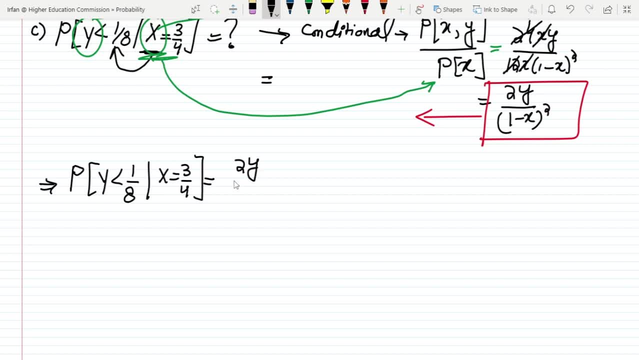 x, which is 3 by 4. so I will get 2 y divided by 1 minus 3 by 4. okay, so this will be squared. okay, so I will get here: 2 y divided by 1 minus 3 by 4 is 1 by 4, so this will become 1 over 16, which will: 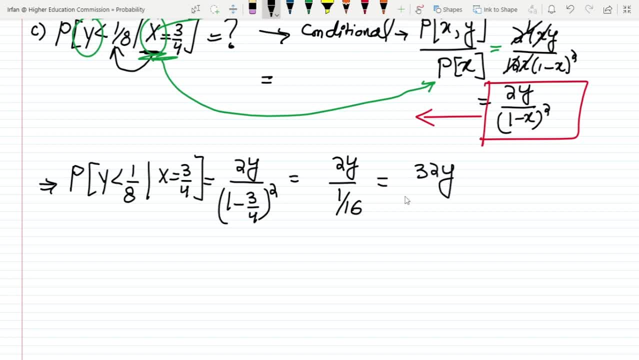 be 32 y. okay, so this is what. this is for the marginal density of this one. okay, so this is for 32 y. and now, in order to find the value for that instance, what we have to do, we have to integrate our value from 0 to 1 by 8. okay, so now integrating it from 0 to 1 by 8, because we are going to find 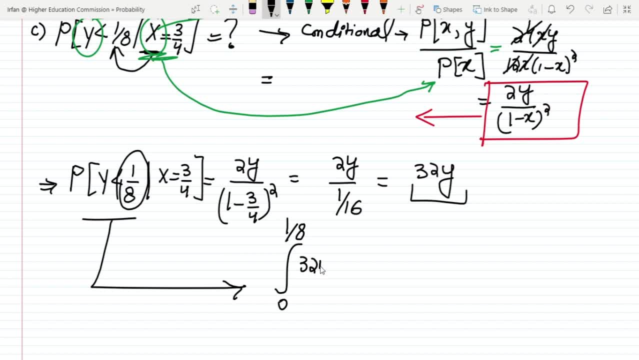 the marginal density. So here it will become 32 y dy. okay, so now it will be 32 into y square, divided by 2, and it will be from 0 to 1 by 8 and ultimately, solving it, what I will get? I will get here 1 by 4, okay, so. 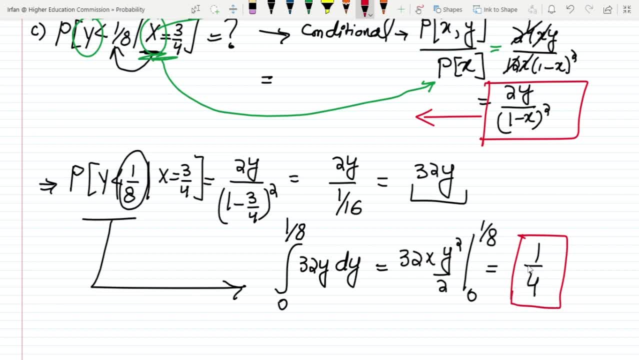 the answer of this is 1 by 4, which we have already found out. okay, so that is basically the solution of part c of my question, in which we have seen that how can we find out the conditional probabilities or conditional density function from any given data? okay, so you have understood that, after finding 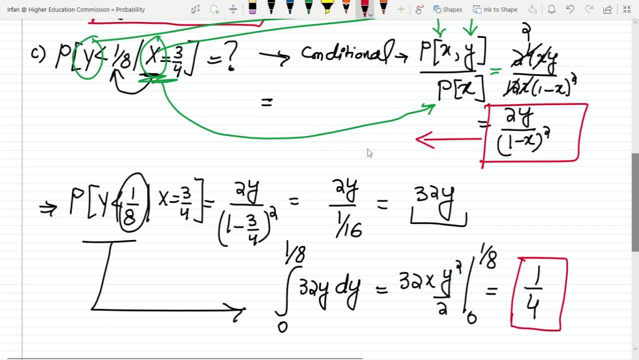 the conditional probability formula from it. I have to integrate it in this range because, no, any restricted range has been defined, but this is the cumulative range and for that I have to integrate it as well. okay, therefore, I had integrated in and the formula given me the answer, which is 1 by 4. okay, so that is it for today, in which we have seen the solution. 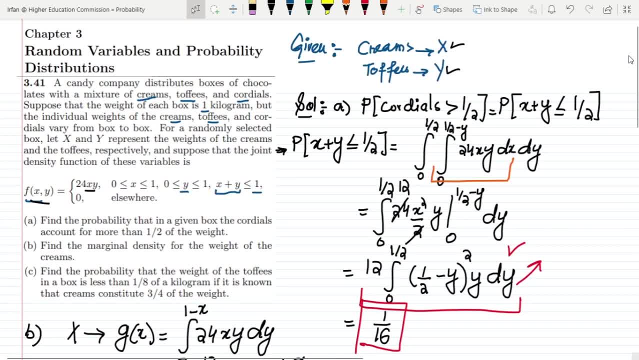 of question 3.41. if you have any question, you can ask me in the comment box. see you soon.